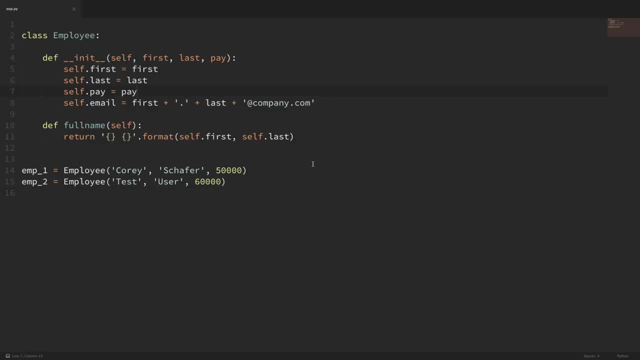 using the self argument that we saw before. So, for example, in the employee class that we created, we set the names, the email and the pay in our init method and those are set for each instance of the employee that we create. And I briefly mentioned class variables in the last video. 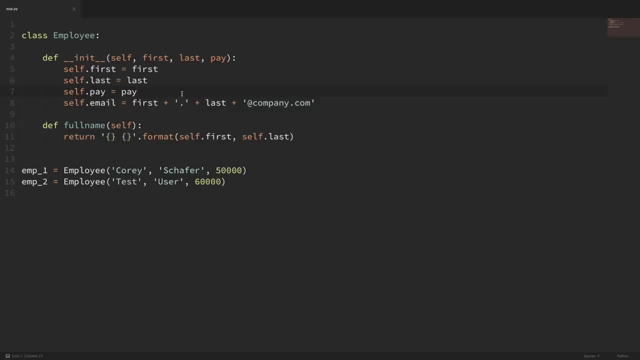 but we didn't go into detail and that's what we're going to learn about in this video. So class variables are variables that are shared among all instances of a class. So while instance variables can be unique for each instance, like our names and email and pay, class variables should be. 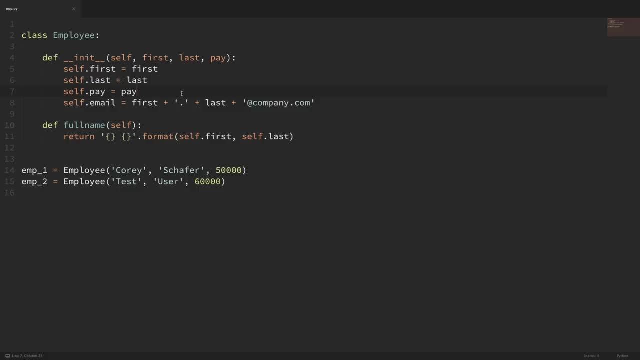 the same for each instance. So if we look here at our employee class, what kind of data would we want to be shared among all employees? So we have a lot of different ideas that we could probably come up with, but for this example, let's say that our 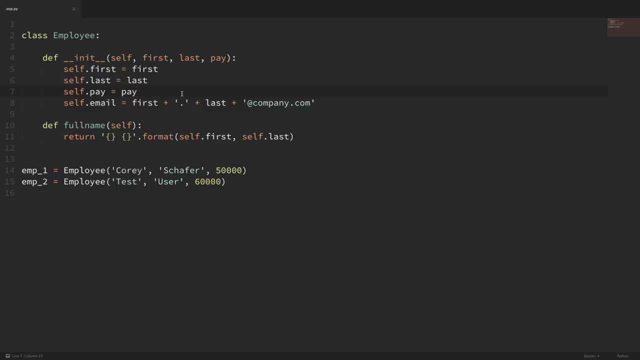 company gives annual raises every year. Now the amount can change from year to year, but whatever that amount is, it's going to be the same for all employees, So that would be a good candidate for a class variable. Now, before we actually create that class variable, let's first hard code this in and see why the class 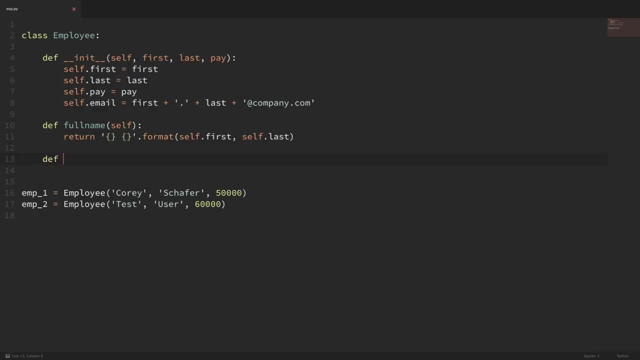 variables would be a better use case. So I'm going to create a method down here called apply- raise and remember our methods Automatically take in the instance which we are going to call self. Now, within this apply raise, I'm going to do a selfpay. 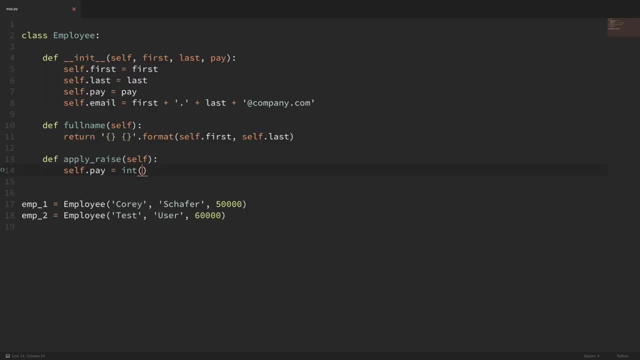 and I'm going to set this equal to an integer, so that we have a whole number, and I'm going to do selfpay times one point, let's just make this four percent. So now, if I was to test this down here on an instance, then I can print out the. 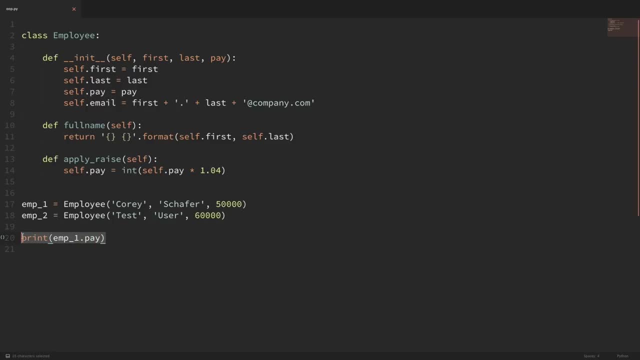 employee one dot pay. and let me go ahead and copy that. I'm going to copy this twice and between here I'm going to do: an employee one dot apply raise. Now, if I go ahead and run this, and I actually forgot to put in the parentheses there. So now, if I go ahead and run this, you can see that I printed out the pay. 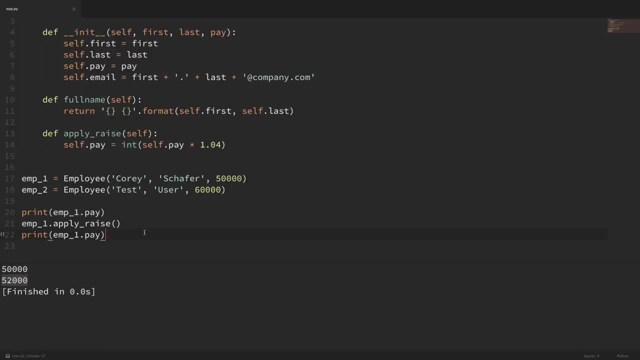 then we applied the raise and it added four percent onto our pay, So we can see that it worked. but there are a couple of things wrong here. So first, it would be nice if we could access the raise amount and then we could go ahead and 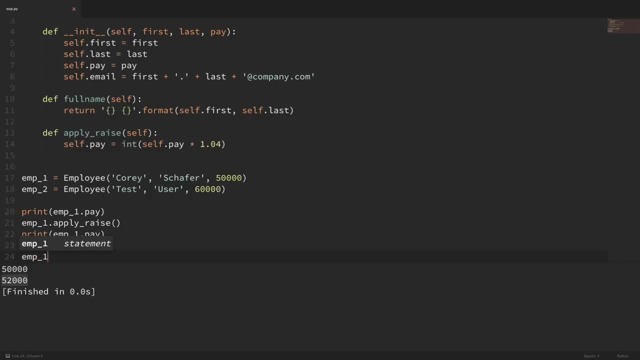 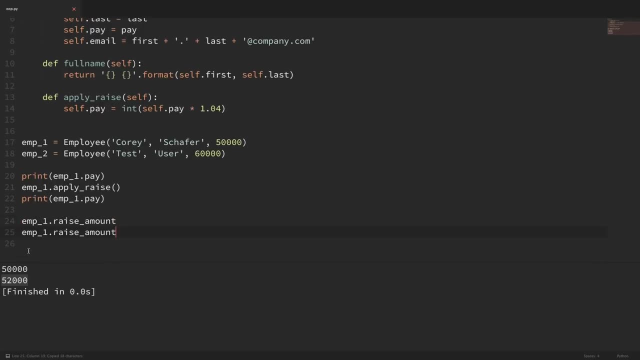 get the raise amount by doing something like employee one dot raise amount or, since it would apply to the entire class, we should also be able to get the raise amount by doing employee dot raise amount. Now that raise amount attribute doesn't currently exist, so we can't see that it is four percent. and also, what if I wanted to easily update that four percent amount? 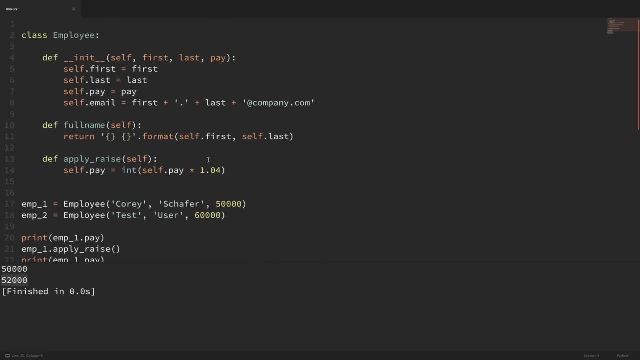 So right now it's kind of hidden within this method And for all I know it could be in multiple places throughout our code. So we don't want to have to manually go in. if we wanted to update this four percent, We wouldn't want to have to manually go in and change these in multiple locations. So instead pull this four. 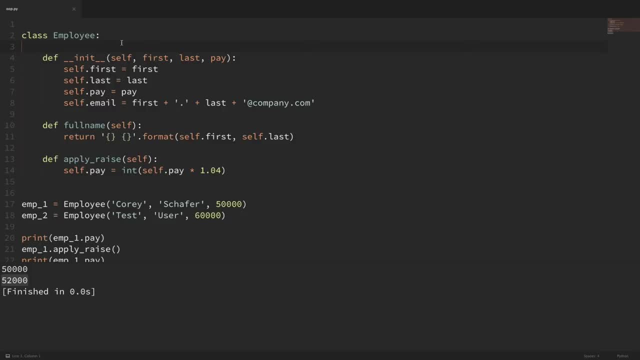 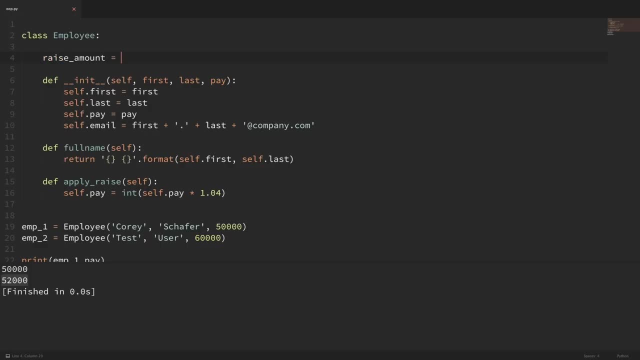 percent out into a class variable, and that's as easy as going up here to the top of the class and just saying that we want a raise amount equal to one point, and we'll just do that at four percent still. So now, instead of hard coding this four percent down here in our apply raise method, Now let's go ahead and use this class variable. 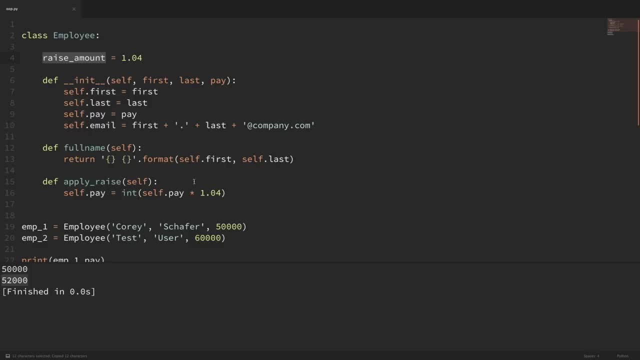 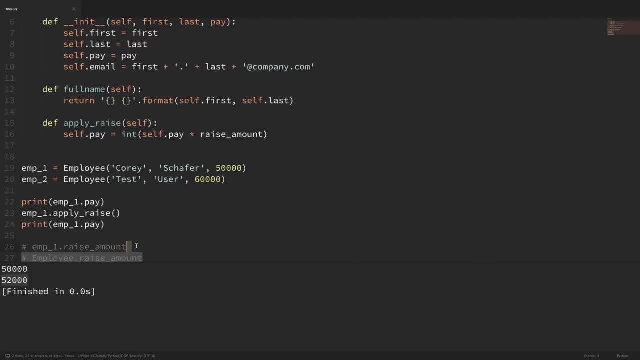 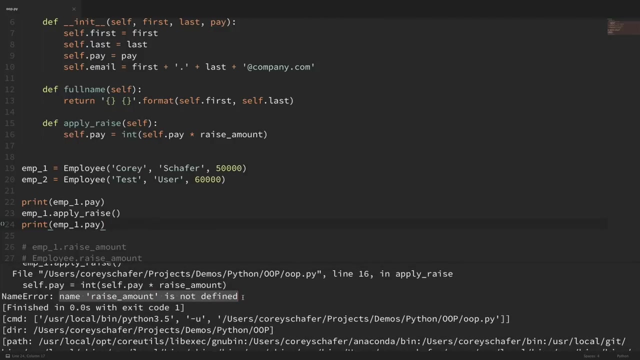 Now you might expect us to just be able to type in raise amount here, But if I save that- and I'm going to comment out these lines here- So if I save that and run it, you can see that I got a name error and it says that raise amount is not defined. And that's because when we access 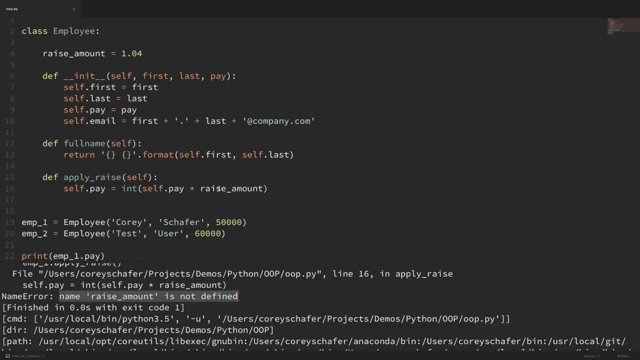 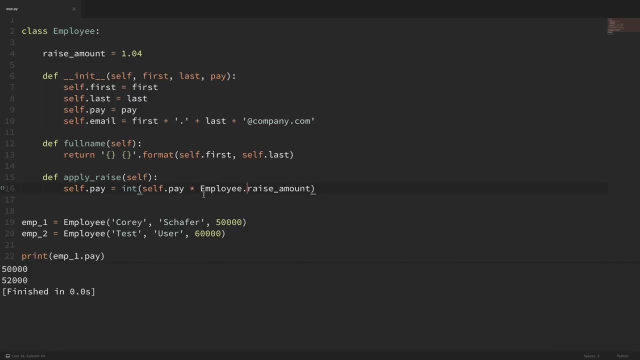 these class variables We need to either access them through the class itself or an instance of the class. So within the apply raise I could either say employee dot raise amount And if I save that and run it then you can see that that works, Or I can also access through the instance. 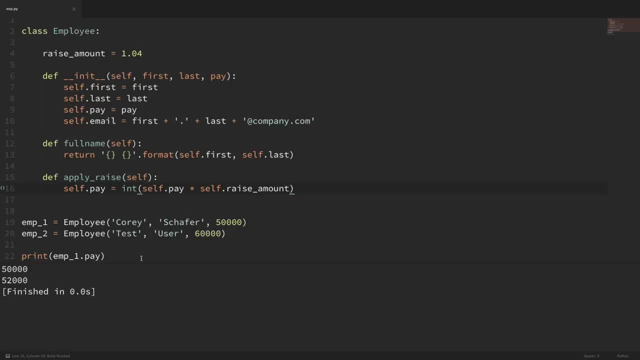 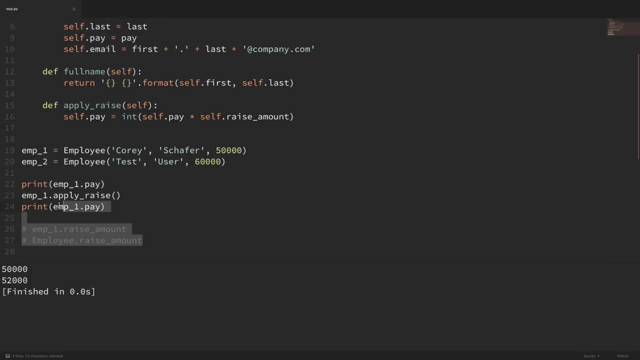 So I can do self dot raise amount, And if I run that then you can see that that works as well. Now that might be a little confusing to you, because if these are class variables, then why can we access them From our instance? So let me print out a few lines here to get a better idea of what's going on. So I'm going to go ahead and remove all of 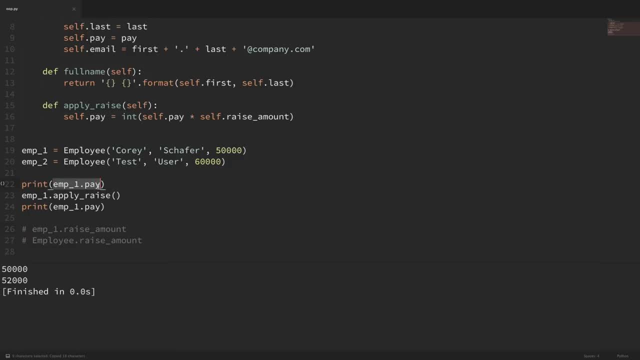 these lines here. Actually, I'm going to keep this And I'm going to print out the employee one dot raise amount And I'm also going to print the employee dot raise amount And also, just to see all of our instances here, I'm going to also do the employee two dot raise. 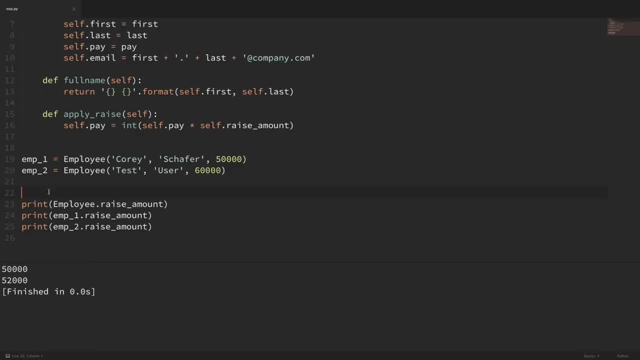 amount so that we can see all of them together. So now, if I go ahead and print these out, You can see that I can access this class variable from both my class itself as well as from both instances. Now what's going on here is that when we try to access an attribute on an 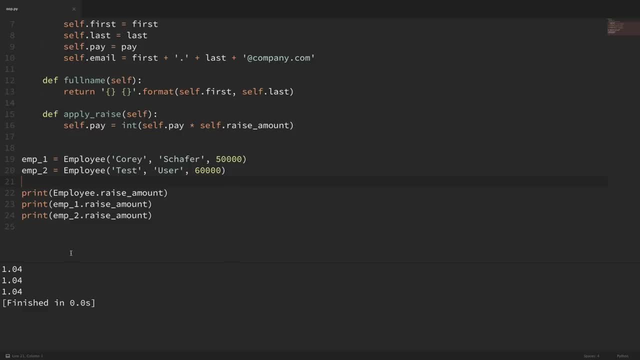 instance. it will first check if the instance contains that attribute And if it doesn't, then it will see if the class or any class that it inherits from contains that attribute. So when we access raise amount from our instances here, they don't actually have that attribute themselves. They're accessing the classes raise. 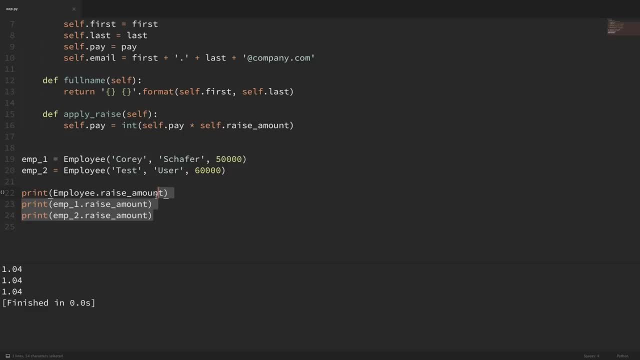 amount attribute. Now there's a little trick that we can do here to get a better idea of what's going on. So I'm going to go ahead and print out the namespace of employee one, And we can do that by printing out employee one double underscore dict. So now, if I run, 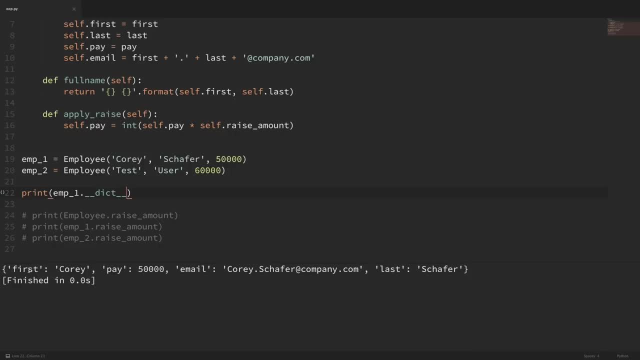 this: if I were to access these names or email or pay, then these are the values that they would return, But you can see that there's no raise amount here in this list. Now, if I printed out the employee dict and run that, Now we're going to get a few things here that we don't necessarily care about. But if we look down here and we can, 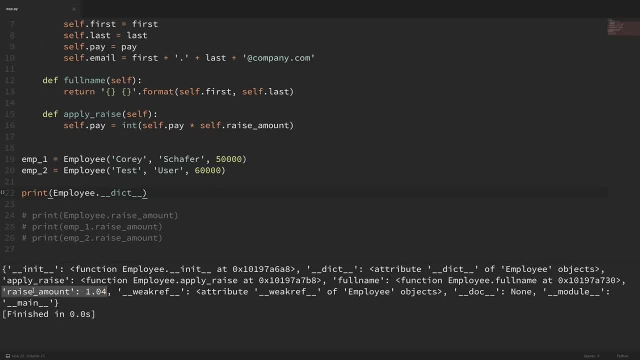 see that the class does contain this raise amount attribute And that is the value that our instances see when we access that raise amount attribute from our instances. Now let me show you an important concept here. So I'm going to go ahead and comment this out and I'm going to take this employee raise amount and I'm going to 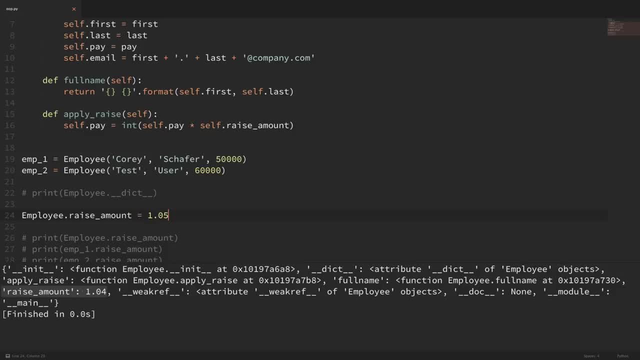 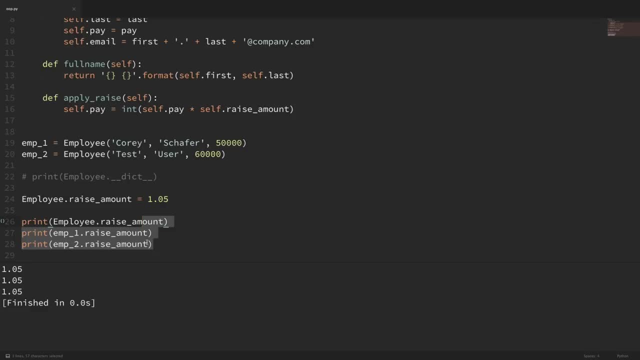 set this equal to 1.05.. And now I'm going to uncomment out our print statements here and rerun this code And you can see that it changed the raise amount for the class and all of the instances. Now what if I was to set the raise amount using an instance instead of using the? 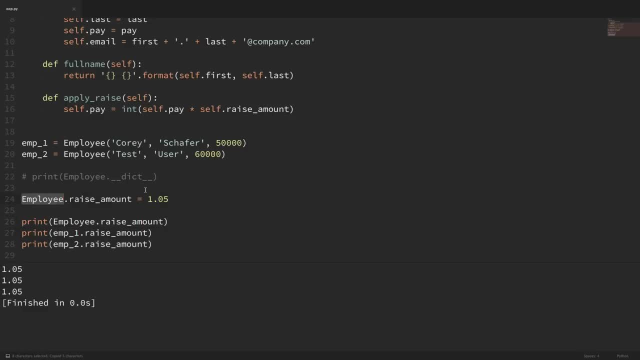 class. So instead of doing employeeraiseAmount equals 5%, I'm going to say employee1.raiseAmount equals 5%. So if I run this now- now this might be a little unexpected- You can see that it only changed the raise amount for employee1.. It's the only one that has this 5%, So why did it do that? 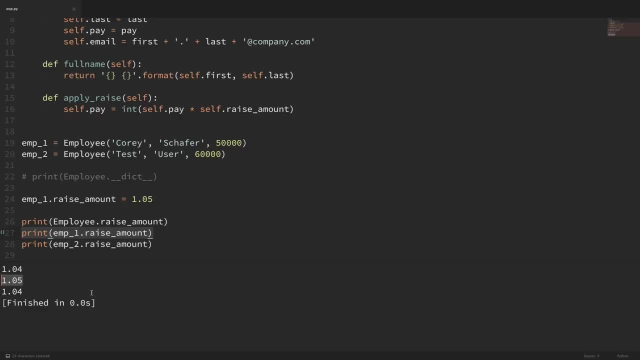 Well, when we made this assignment, it actually created the raise amount attribute within employee1.. So if I go back up here and print back out employee1's namespace- and I'm going to do this under the assignment- So now, if I run that now, you can see that employee1 has raise amount within its. 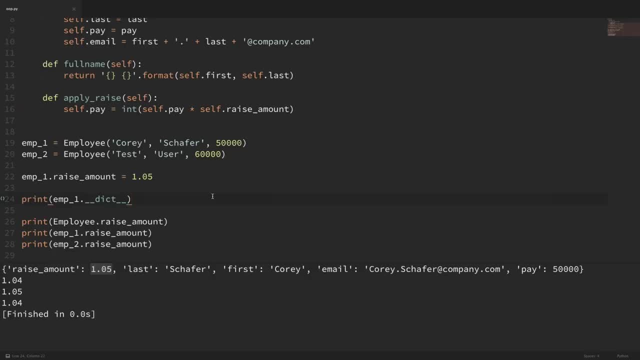 namespace equal to 5%, And it finds this within its own namespace and returns that value. So in this case it doesn't have to happen. What I did here was I did a set up what is called a raise amount, which is an attribute that's using the class's value before going and searching the 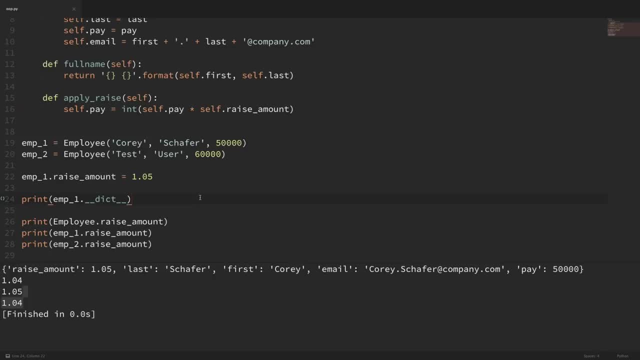 class and we didn't set that raise amount on employee2, so that still falls back to the class's value. Now, that's an important concept to understand, because up here in our applyraise method we can see that we could get different results depending on whether we did the self. 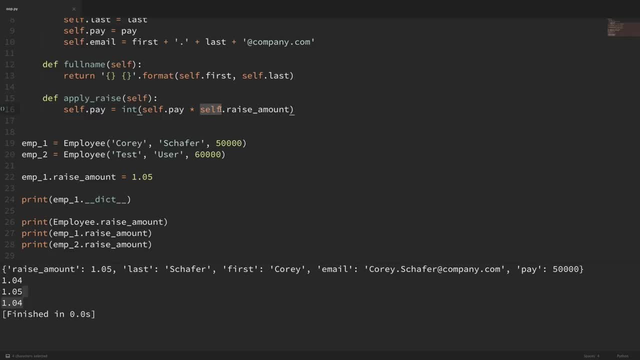 which is the instance raise amount, and leave this as selfraiseAmount, because that will give us the ability to change that amount for a single instance if we really wanted to. So if I wanted to change employee1's raise amount, then I could go ahead and do that And when I did apply raise then it would use the employee1's 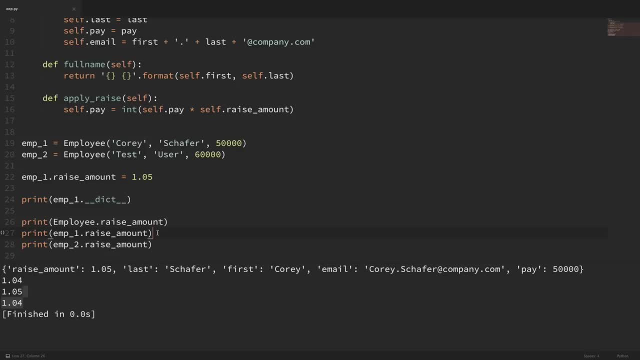 raise amount instead of the class's raise amount, And also using self here will allow any subclass to override that constant if they wanted to, And we'll look at subclassing in a future video. So now let's look at another example of a class variable where it wouldn't really make sense to 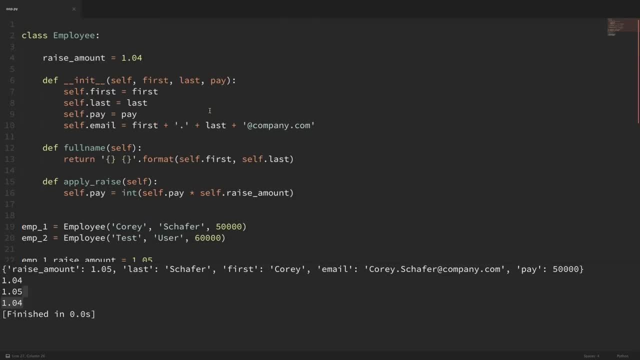 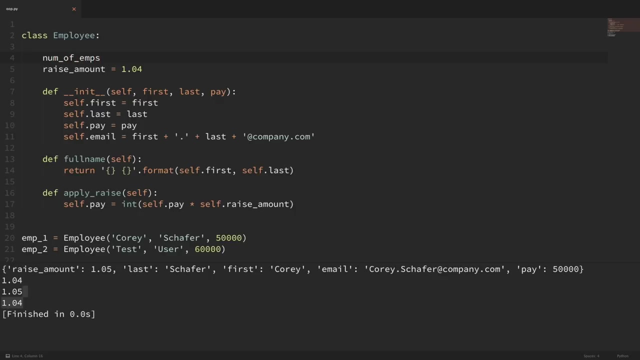 use self. So let's say that we wanted to keep track of how many employees that we have. So the number of employees should be the same for all instances of our class. So if I created a class variable up here, I'm just going to go ahead and call this: numOfEmployees is equal to. 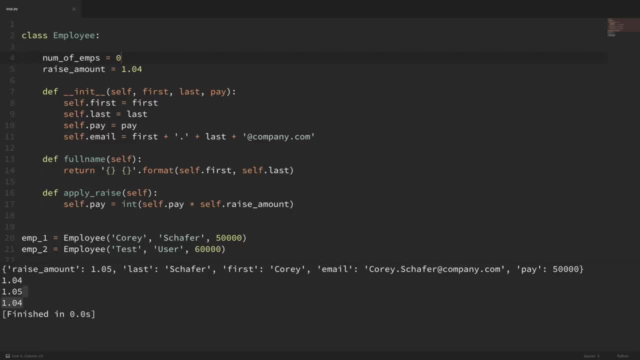 zero for now, And each time we create a new employee I'm going to increment that by one, And I can do that within the init method, since the init method runs every time we create a new employee. So within here I'm going to do: employeenumberOfEmployees plus equals one. 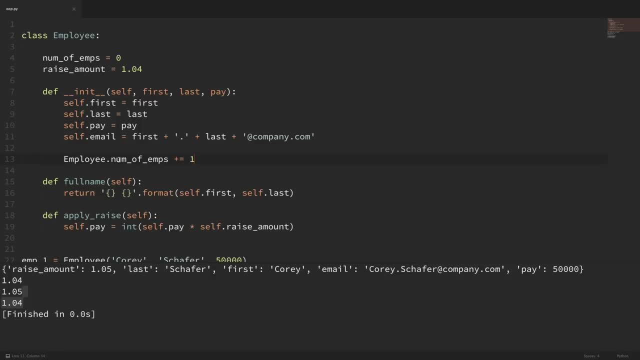 Now I'm definitely going to use employeenumberOfEmployees here instead of selfnumberOfEmployees, because with the raise amount I'm going to use selfnumberOfEmployees And I'm going to do create a new employee and then I'm going to say emploinumberOfEmployees, And so this is. 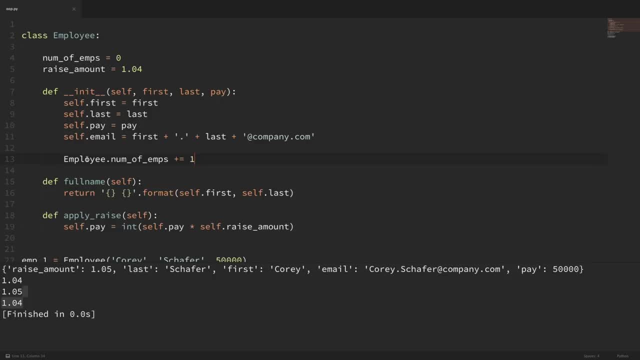 where we're going to use the numOfEmployees, So that's what we're going to use. So for now, I'm going to go ahead and go ahead and delete all of these cases. It's nice to have that constant class value that can be overridden, per instance, if we really need it to be. But in this case, 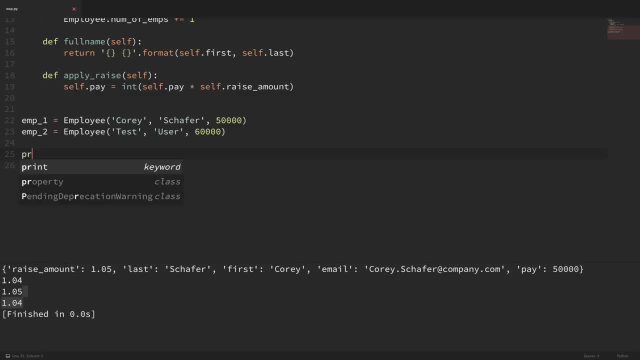 there's no use case. I can think of where we would want our total number of employees to be different for any one instance. So for now I'm going to go down here to the bottom And go ahead. you can see that it returned two because it was incremented twice when we instantiated both of our 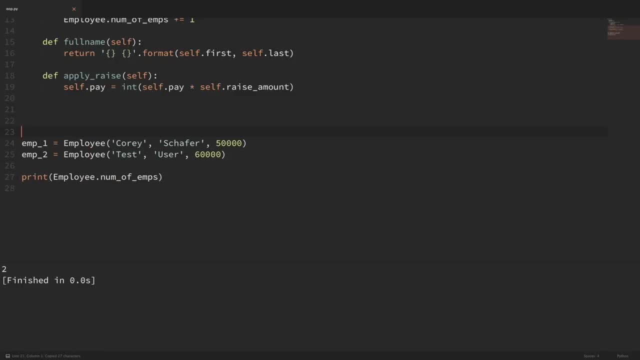 employees here. If I was to put this print statement above, where we instantiated those employees, then you can see that it was zero and we created two employees and then it printed out two. Okay, so I think that is going to do it for this video. Now, I know that that was a lot to. 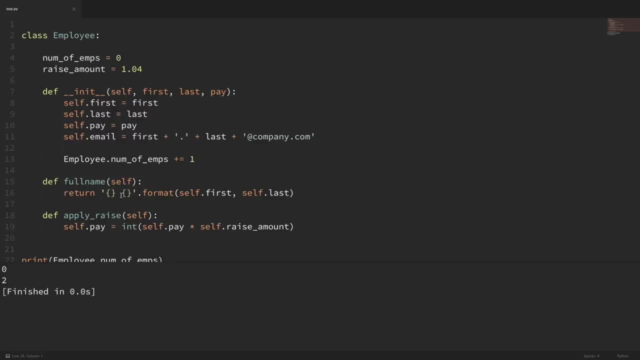 take in. but hopefully now you better understand the difference between instance variables and class variables and when you would use each one. So one of the obvious next questions is: well, if we have class variables, then are there also class methods? And the answer is yes, There are. 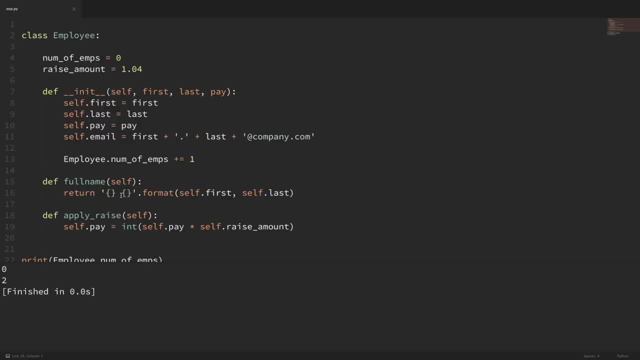 these things called static methods and also class methods, and we'll look at the difference between those in the next video. But if you do have any questions about what we covered here, then feel free to ask in the comment section below and I'll do my best to answer those If you enjoy these. 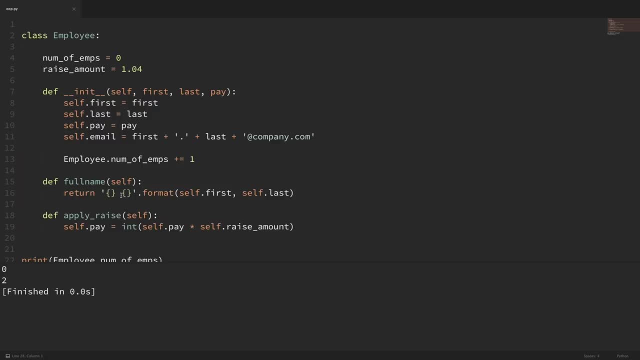 tutorials and would like to support them, then there are several ways you can do that. The easiest way is to simply like the video And give it a thumbs up, And also it's a huge help to share these videos with anyone who you think. 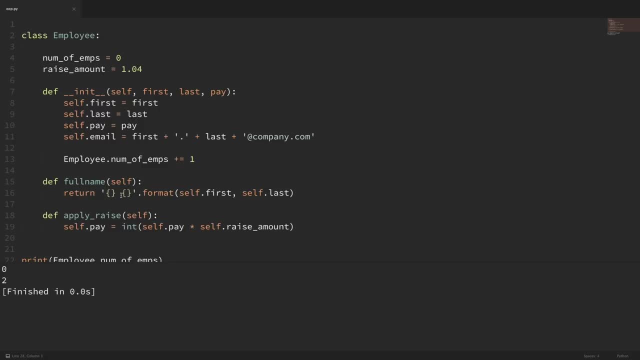 would find them useful And if you have the means, you can contribute through Patreon, and there's a link to that page in the description section below. Be sure to subscribe for future videos and thank you all for watching.